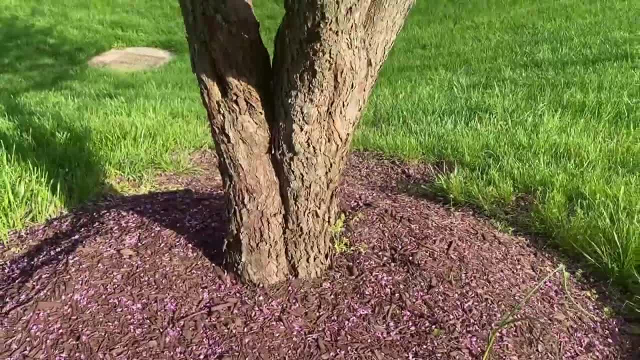 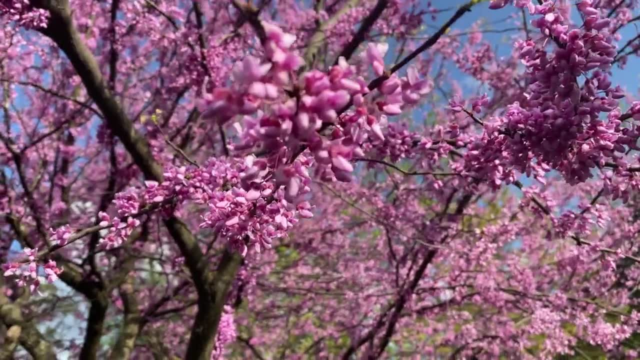 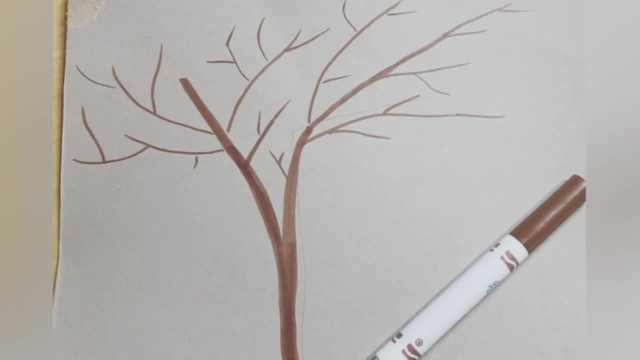 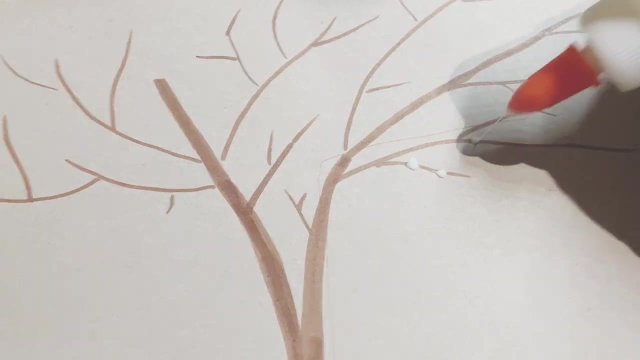 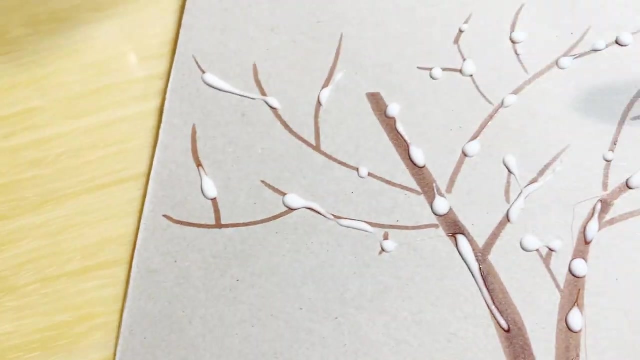 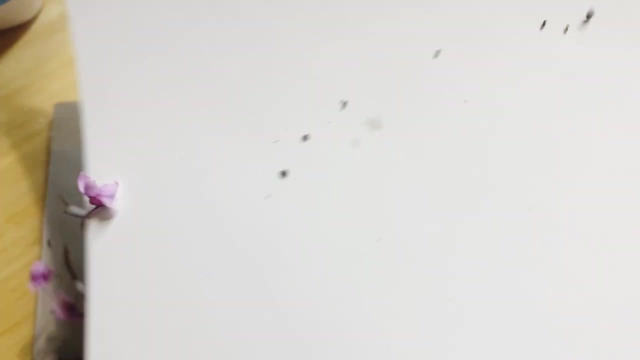 My favorite part of spring is seeing the flowers, the flowering trees. sadly, they are falling off now, but don't worry, here's an activity that will revive those trees. here I made a tree and branches with a brown marker, then I added glue and sprinkled the redbud flower just like glitter feel. 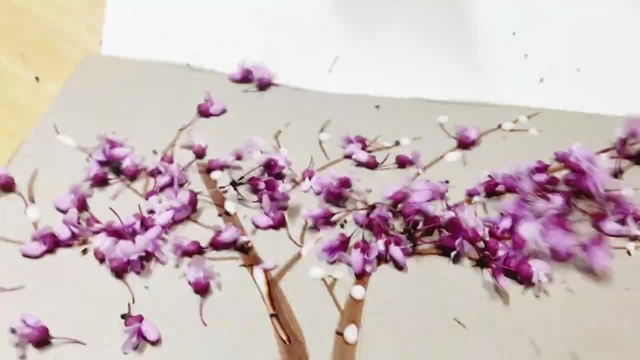 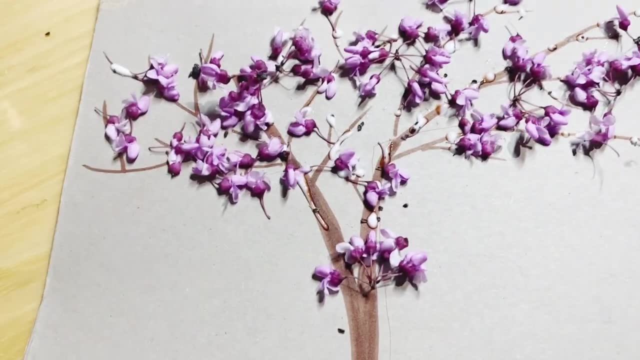 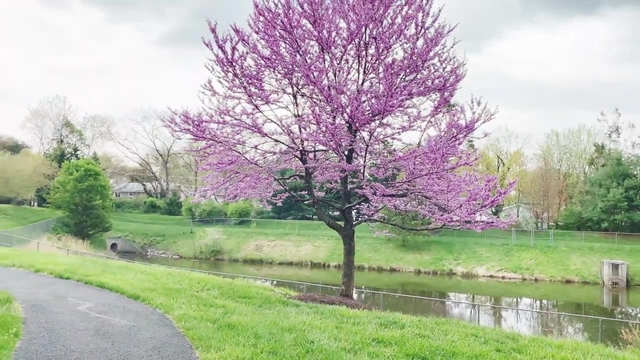 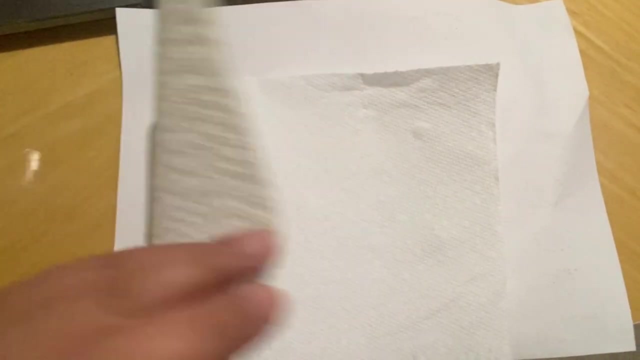 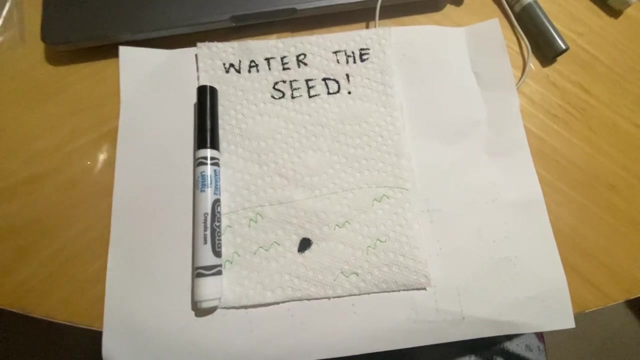 free to use whatever flower is in season, but if you miss the flowers, then you can try using leaves instead. and there you have it: an indoor redbud tree. in the next one I have a paper towel and I fold it in half. on the outer side I wrote water the seed and drew a 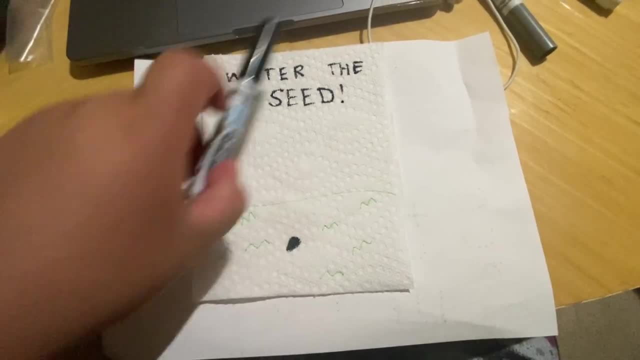 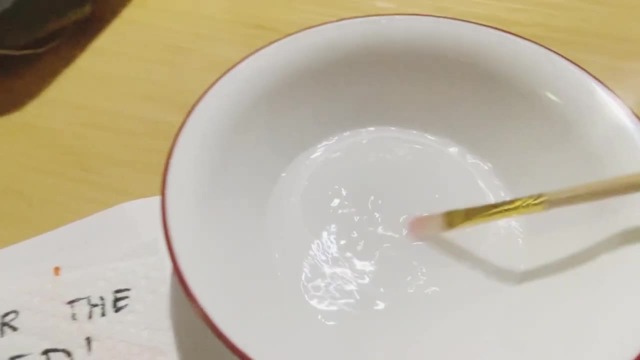 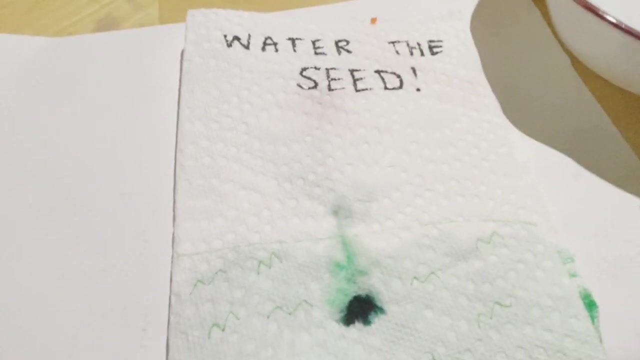 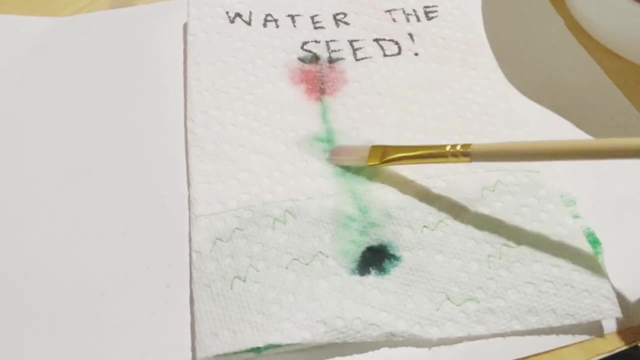 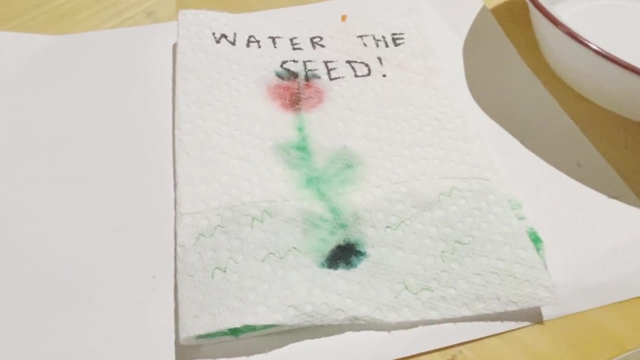 small oval for a seed and then on the inner part I drew a flower. then I took a paintbrush and painted water over it until the flower bloomed. you would have the same result if you threw the paper towel in a bucket of water, but that's just too quick and it encourages me to use more paper towel. 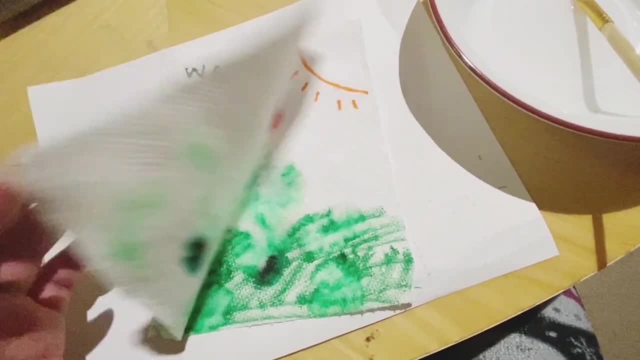 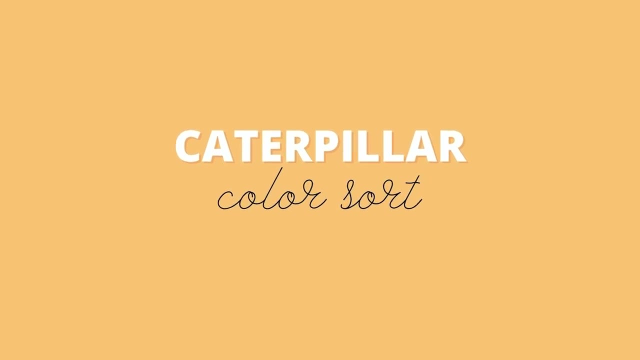 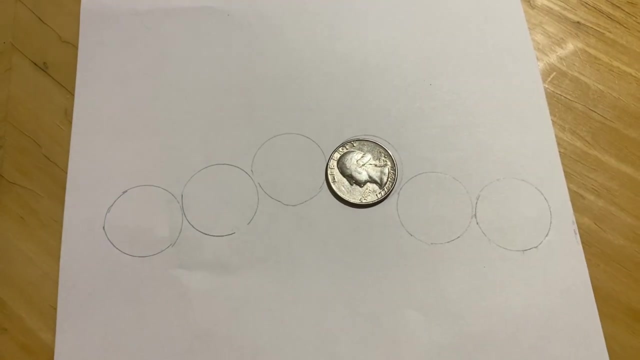 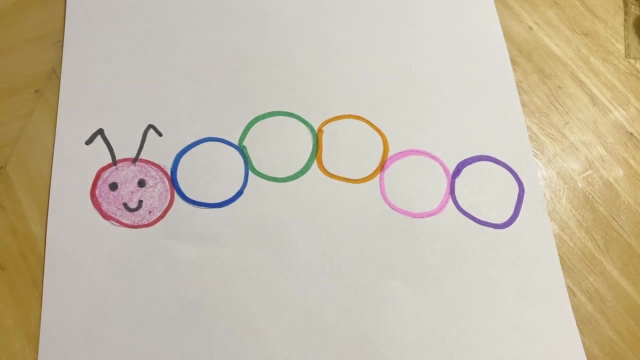 you. the last activity can be messy, so make sure you have something underneath. the last activity will help develop fine motor skills and color recognition. here I used a quarter and traced it to form a caterpillar. I then used a marker to outline the circle. next I got a zip lock bag and 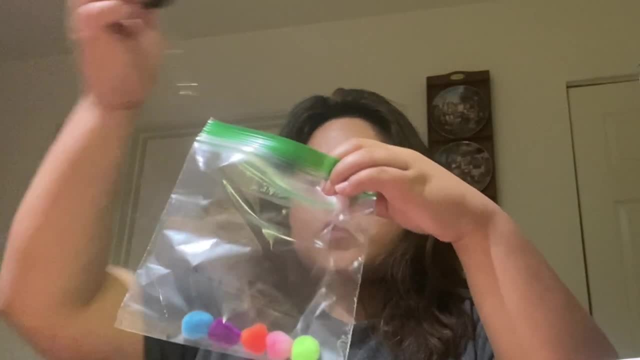 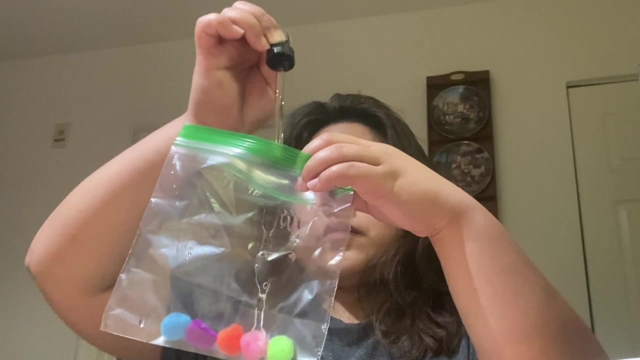 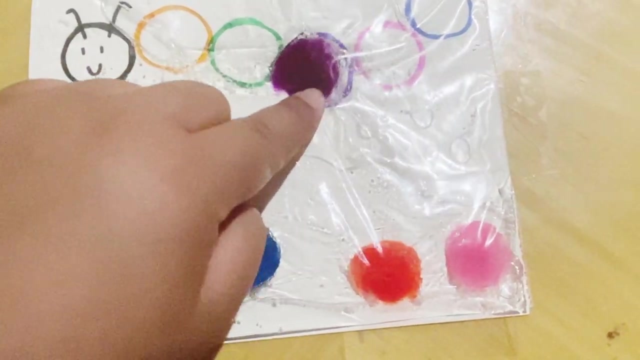 added pom-poms and oil. you can use baby oil or cooking oil oil. I then tape the drawing onto the table, then tape the ziplock over it. To be clear, the drawing is not inside the ziplock, it's just under it. Make sure to.